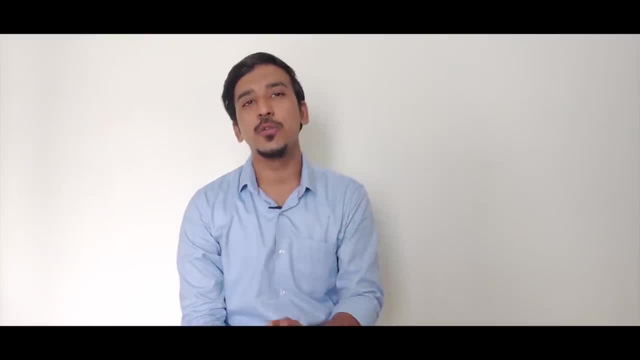 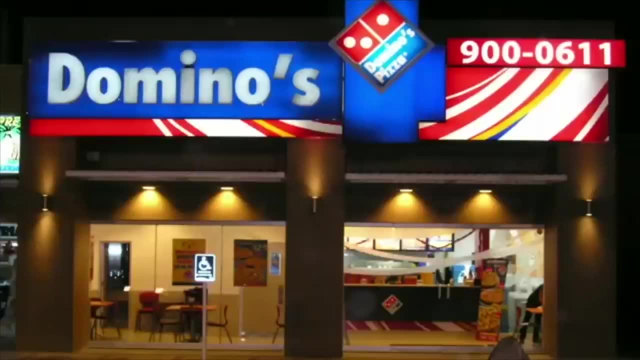 This is a story that dates back to 2009,, when the brand image of Domino's was completely down the drain. The stock was selling at a rate of 1.5% at a rock bottom price of just $6 per share. The store sales were going down drastically. 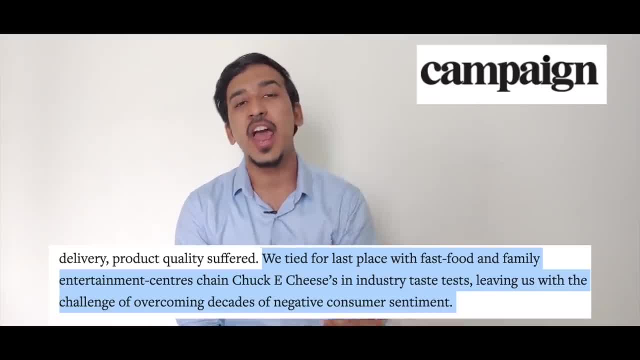 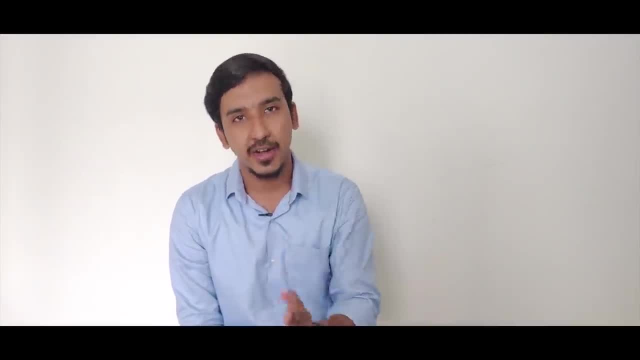 and Domino's ranked last in the Consumer Brand Preference Survey. All of these things made it very, very clear that Domino's was failing real bad. This is when the CEO of the company back then, Patrick Doyle, decided to take a closer look at the situation. 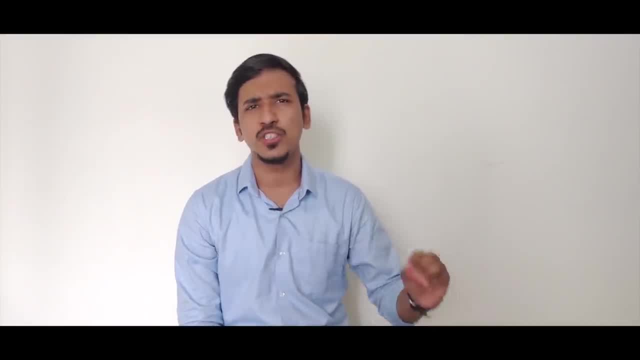 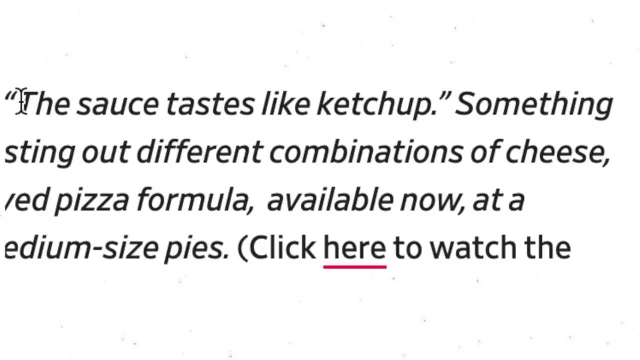 And soon enough, they found out that there were multiple blog posts saying how bad their pizzas were. Some of them said that the crust of the pizza tasted like cardamom, While the other said that the sauce tasted like ketchup, And this was followed by a series of social media posts. 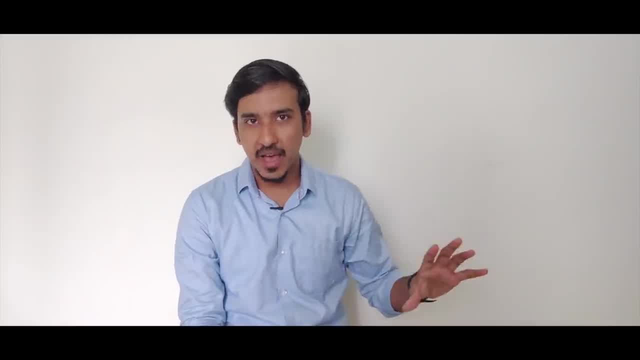 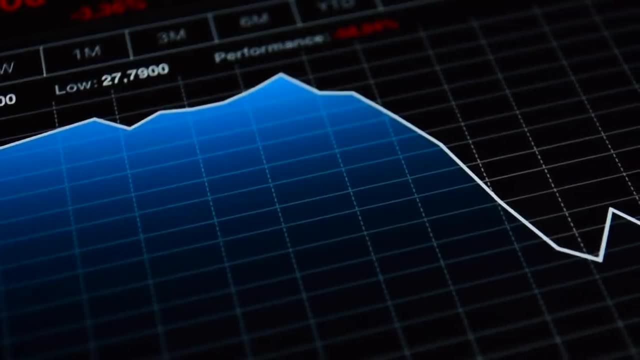 which consistently appeared online. Now, if you take a step back and try to understand the situation, the situation is very, very delicate. The stock price of Domino's was already hitting a rock bottom. The American economy was still recovering from the 2008 crisis. 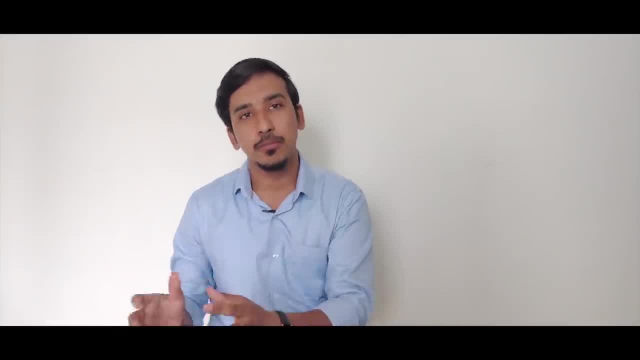 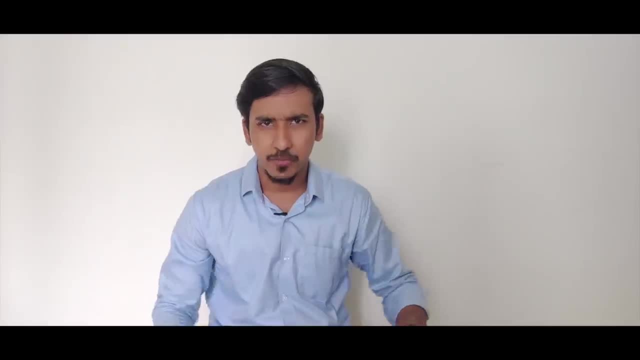 And during this time, Domino's, as a publicly listed company, was already walking on a very, very tight rope. Now, in this case, what any normal company would do is they would engage in great PR. they would make sure that all the bad reviews are overshadowed. 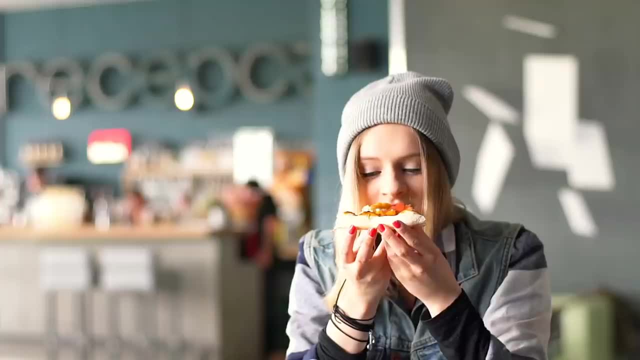 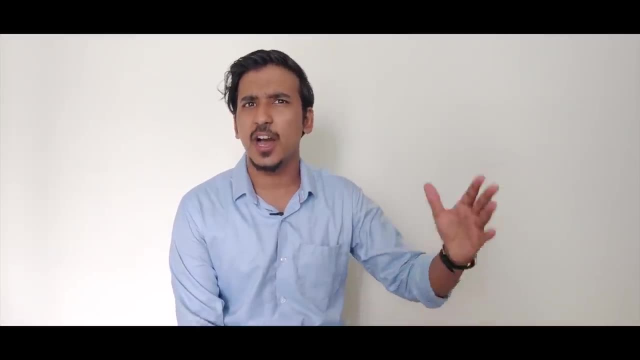 and then, in the background, they would make a few changes and maybe even give out free pizzas just to get positive reviews. Or, worst case, they would just ignore this altogether, thinking that after all, in 2009,, what could a blog do to a billion dollar company? 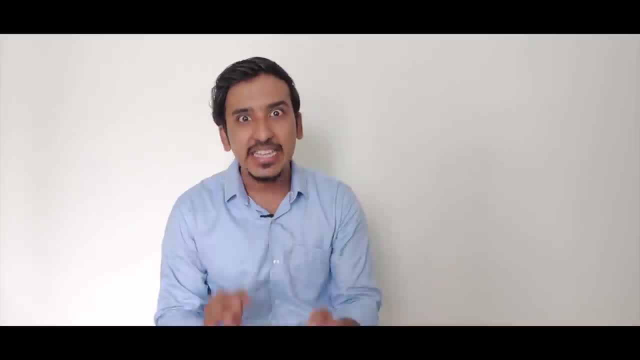 But you know what? Domino's opted for the most lethal weapon in advertising That nobody ever dares to use, especially when the company is failing, And this weapon was brutal honesty. Patrick Doyle, the CEO of the company, took full responsibility of what was happening. 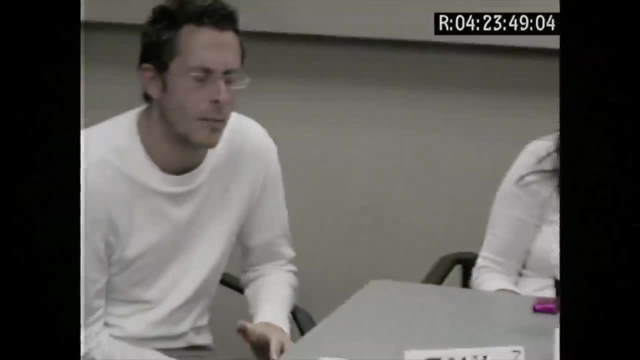 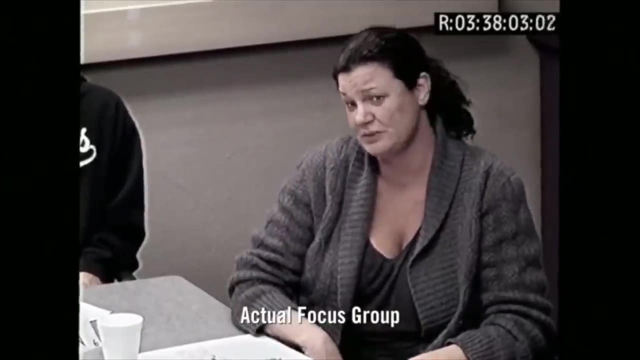 and he publicly admitted that they were not doing a good job. In fact, they called upon actually disappointed customers and got them to taste the pizzas to give them feedback. And it was perhaps the most difficult day at work, because every person who walked in just put out some brutal phrases. 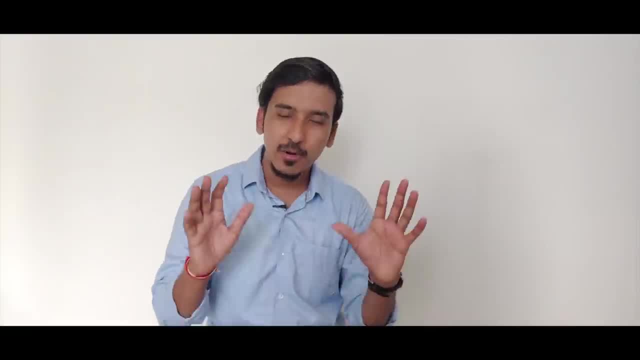 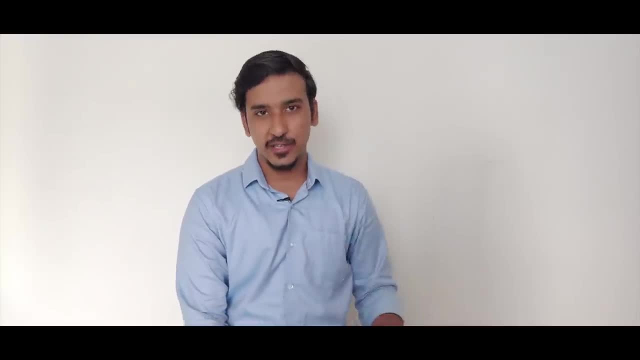 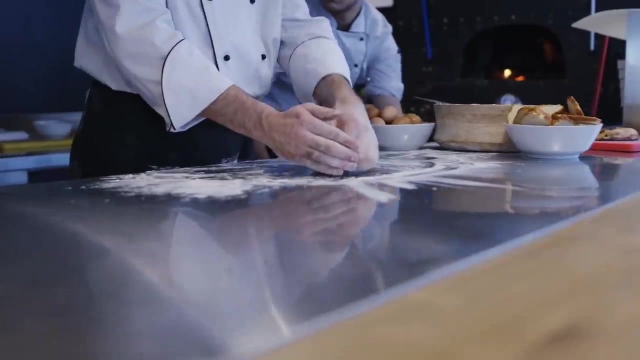 and told them how pathetic their pizzas were. But the team of Domino's listened to them very, very patiently and took notes diligently. But what followed next was nothing short of an adventure. For the next 18 months, every single chef of Domino's worked day in and day out. 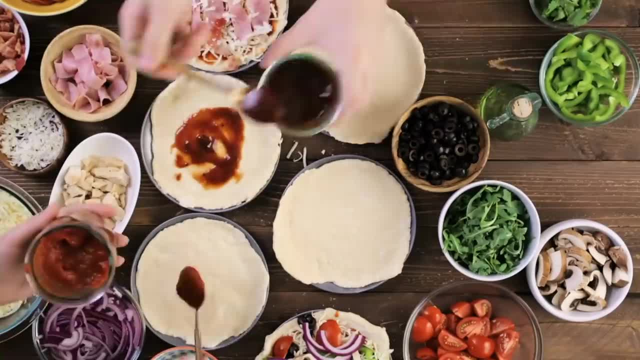 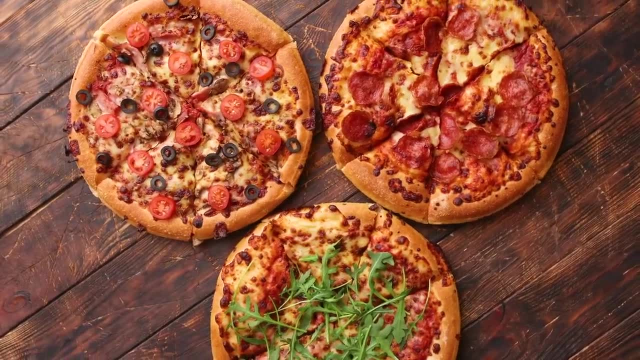 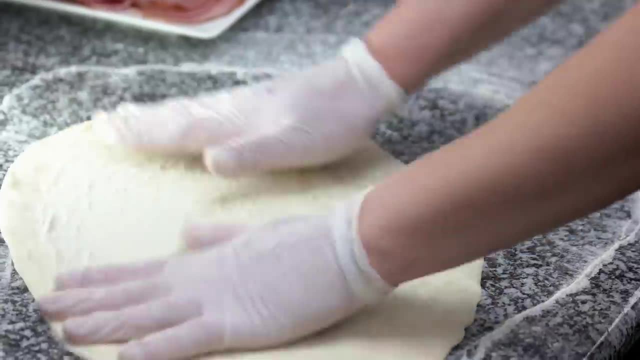 without taking a weekend off just to try every possible combination of ingredients to make the best pizzas they possibly can. And they changed their pizzas from top to bottom. And in the process of this experimentation, they also realised the fact that, in the race of actually providing customers with 30 minutes delivery, 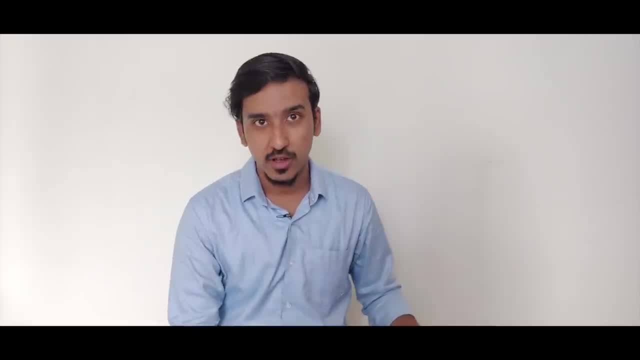 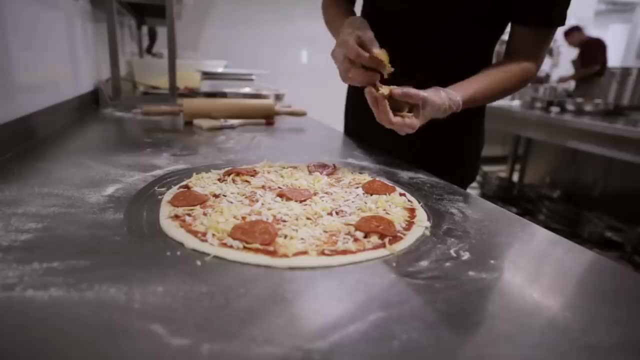 the company's supply chain itself was compromised. The majority of its ingredients were frozen, canned and even pre-made, just so that they could cut down on cost and to make it easier to assemble a pizza in a record time. So the chefs and the management got together. 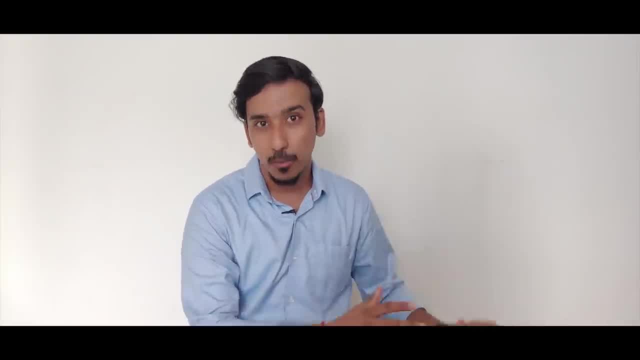 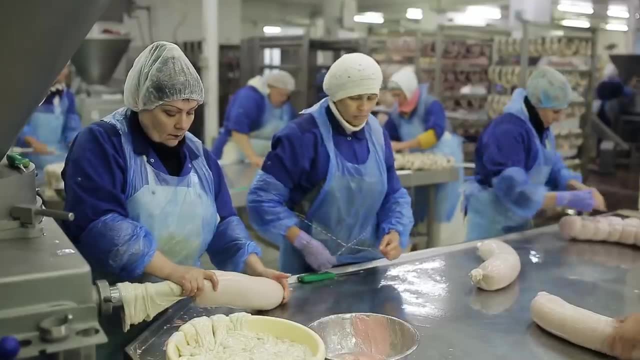 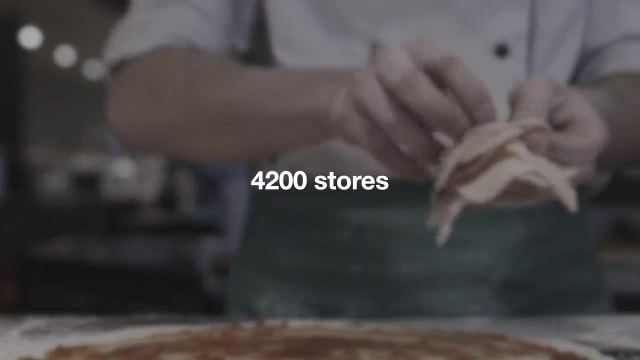 and changed the entire supply chain of the company. Now, this was an extraordinary move because we are looking at a complete revamp of processing, inventory, storage and transportation that is going to be executed to a chain of more than 4200 stores which are spread across 9.93 million square kilometers. 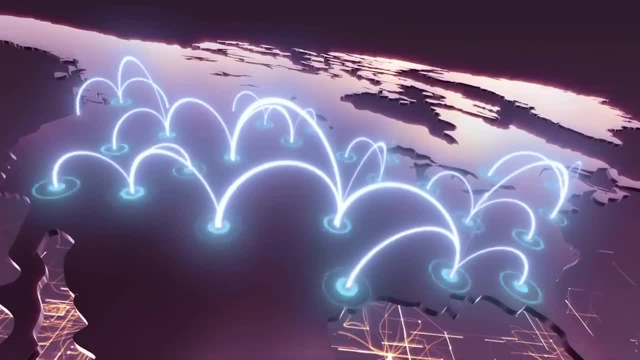 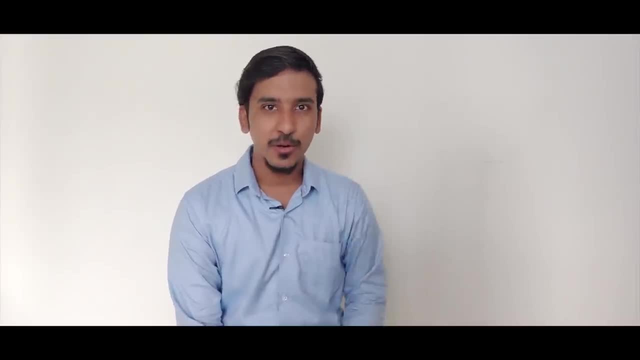 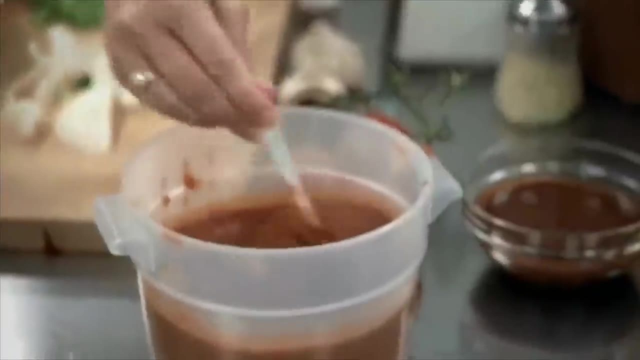 which is practically three times the size of India. But to everyone's surprise, they managed to pull it off within just 18 months. And guess what? On top of that, they launched a campaign called Oh Yes, We Did It campaign, wherein they documented their entire journey of how they went from making terrible pizzas 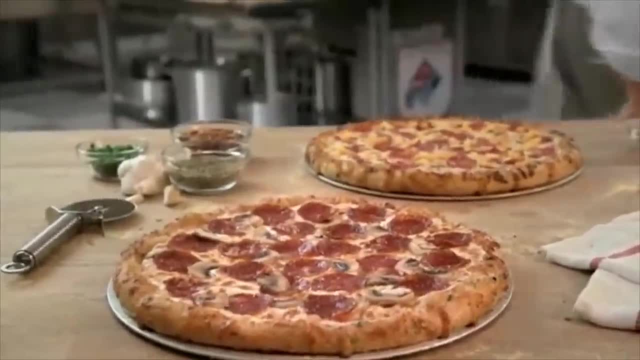 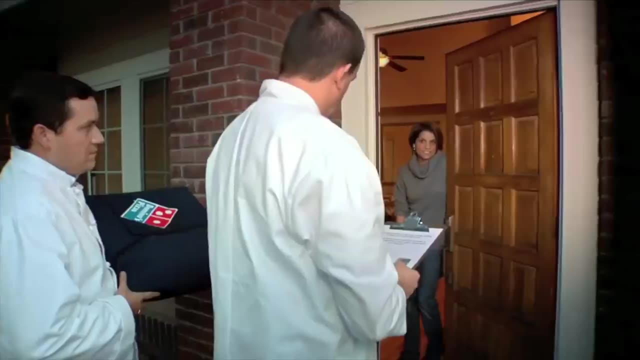 to making the best pizzas in the United States. In fact, there is also a very sweet video online wherein the head chefs of Domino's personally go to the houses of their harshest critics and they surprise them with their new pizza, wherein they had incorporated all of their feedback. 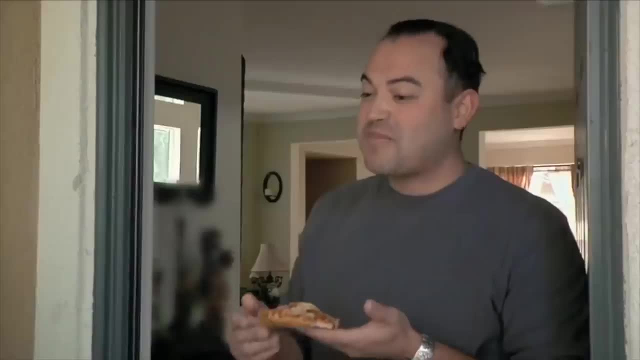 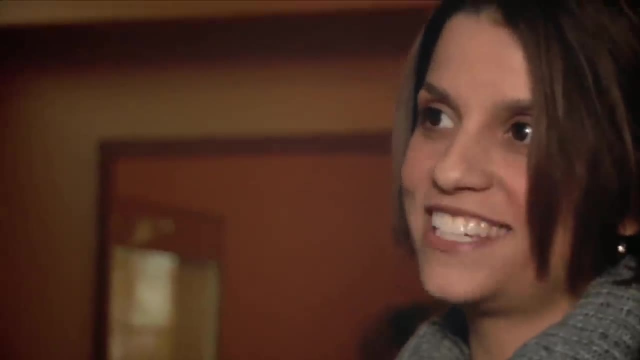 And each one of these critics was mind blown that the head chef of Domino's himself had come down to deliver pizzas. They tasted the pizzas, they loved it and they were smiling, and most of them couldn't even believe that such a huge company would actually take their feedback so seriously. 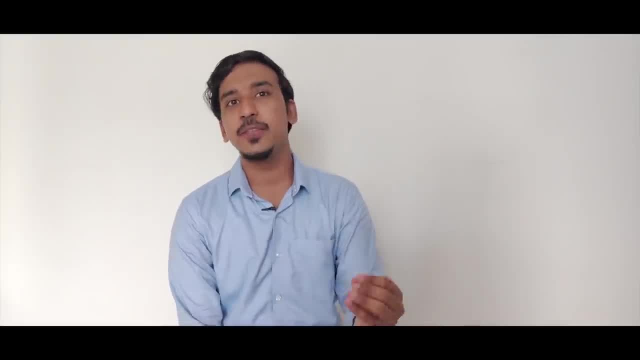 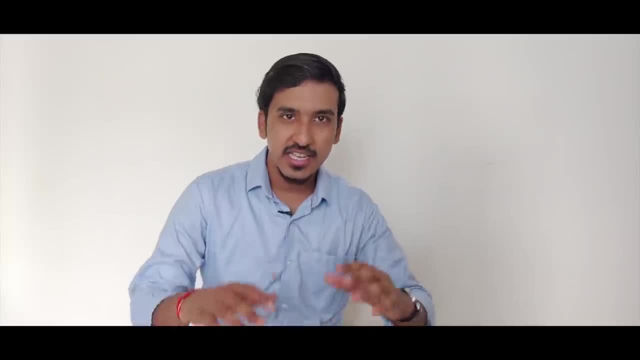 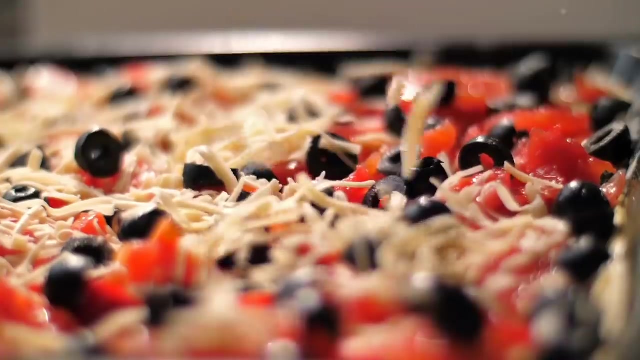 Apart from this, they also included a special section in the website wherein they featured Facebook posts and tweets of customers who expressed their delight after having their new pizzas. This is how Domino's reinvented itself and did everything in its capacity to get back to making the best pizzas in the United States. 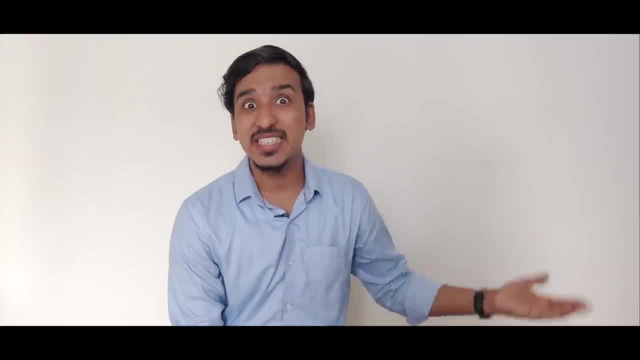 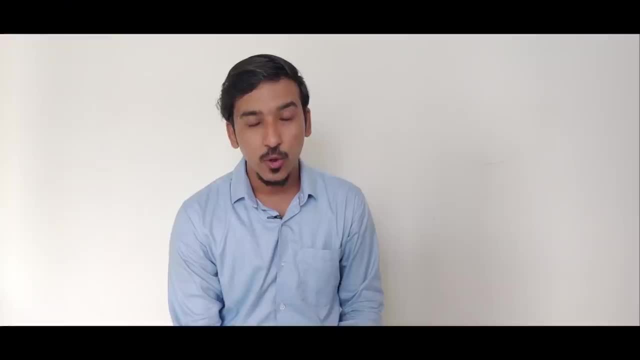 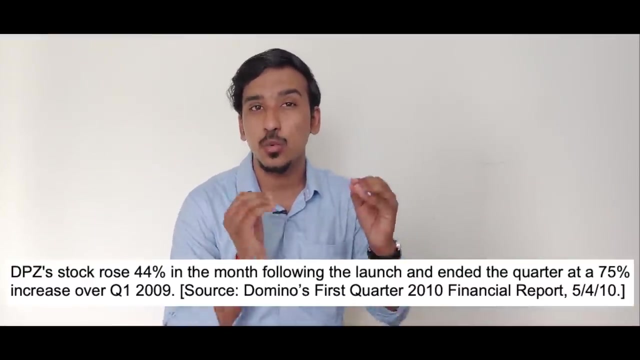 And the results? Well, while the pizza delivery business itself saw a decline of 3%, the same store sales of Domino's rose by 14.3%, which is the largest quarterly increase in fast food history. The Domino's stock rose by 41% in just one month following the campaign. 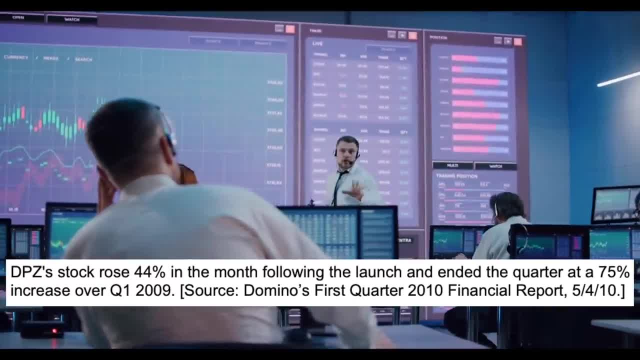 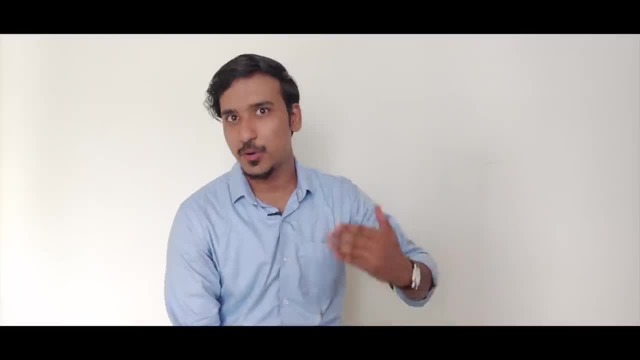 and by the end of the quarter the stock had reached 75% increase. The campaign has earned 2 billion dollars. The campaign has earned 2 billion dollars. The campaign has earned 2 billion free media impressions till date and the stock price just kept going and going for 7 years. 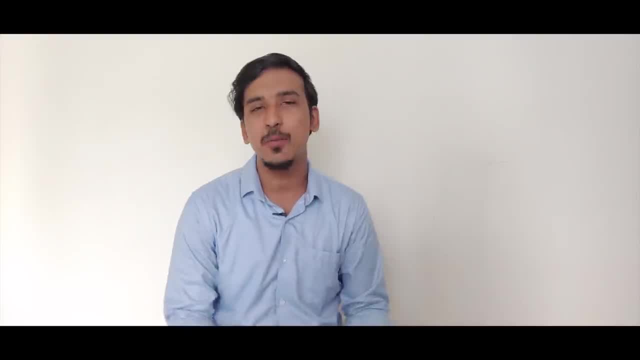 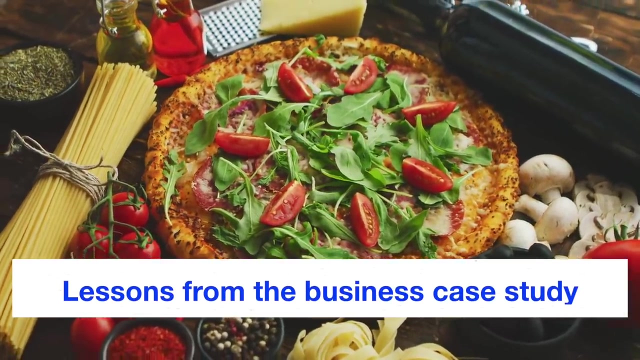 and rose by 2000%, outperforming Apple, Amazon and Netflix. This is how Domino's set a benchmark for other brands to learn on how to embrace criticism and how to turn it into a business opportunity. Now there are 3 very important lessons that we need to learn from this case study. 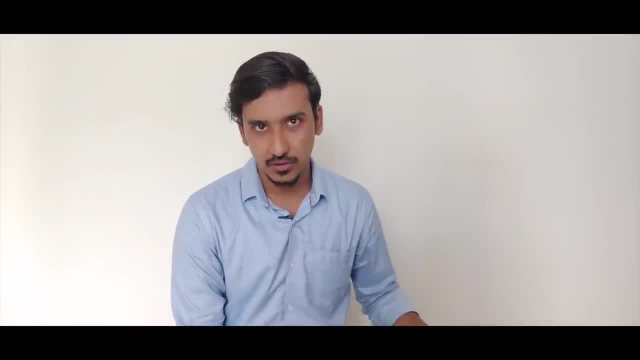 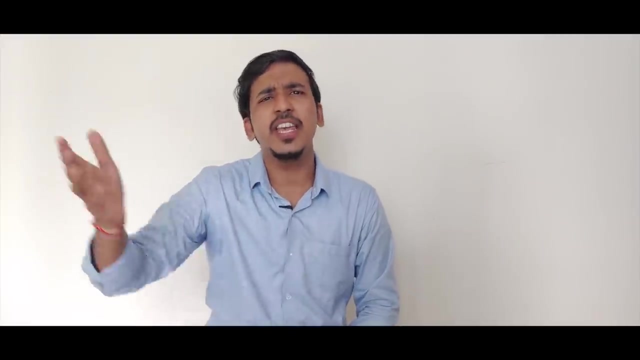 Lesson number 1: Customer criticism is a part of the business, although sometimes there might be meaningless hate. as a business owner, it is your responsibility to filter through the chaos and identify the weakness before it paralyzes your business. In this case, the CEO could have easily ignored the blocks. 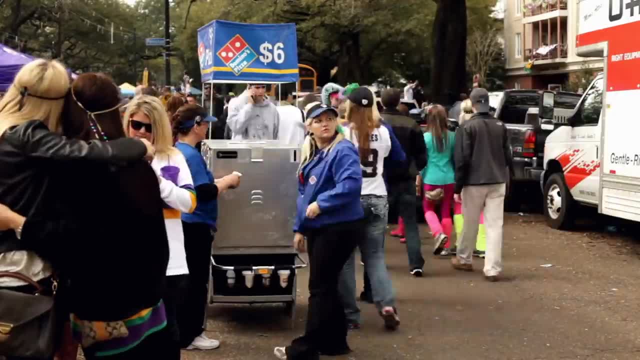 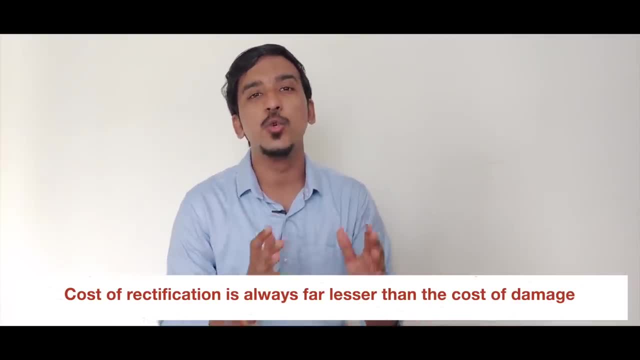 but because he decided to fix it, Domino's still exists. Lesson number 2: The cost of rectifying a mistake is always far less than paying the price for it when it's already too late. In this case, if Domino's had considered revamping the supply chain to be a million dollar export. 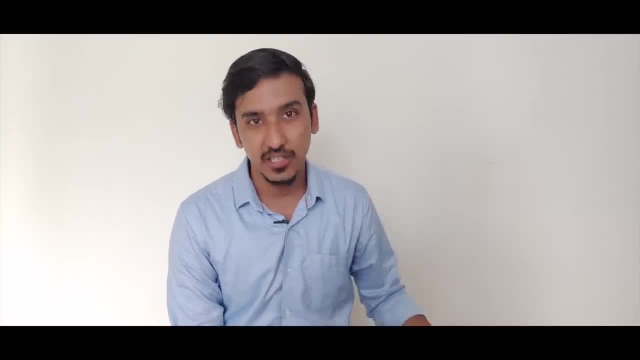 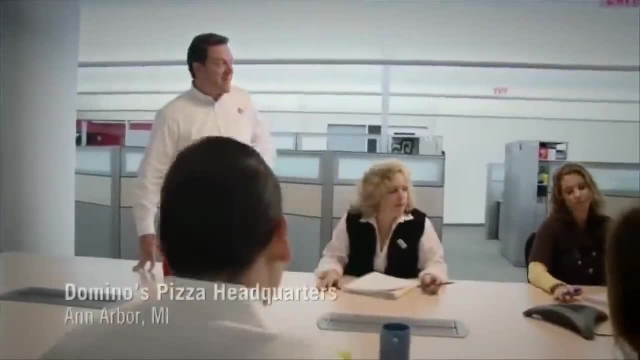 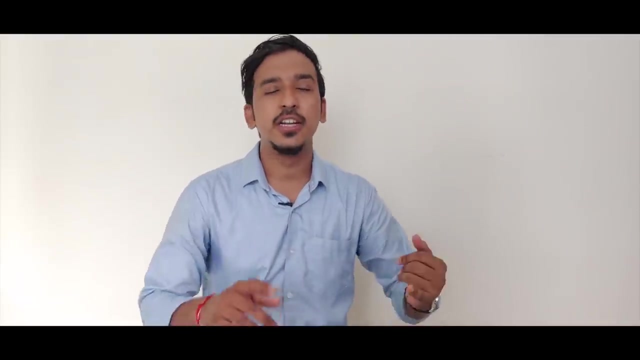 it would have cost them their entire business, But because they saw it as a million dollar investment, it gave them the opportunity to rise from their ashes. And, last and most importantly, every brand needs to realize that the future of marketing is not about discounts and fancy packaging, Although they are important. 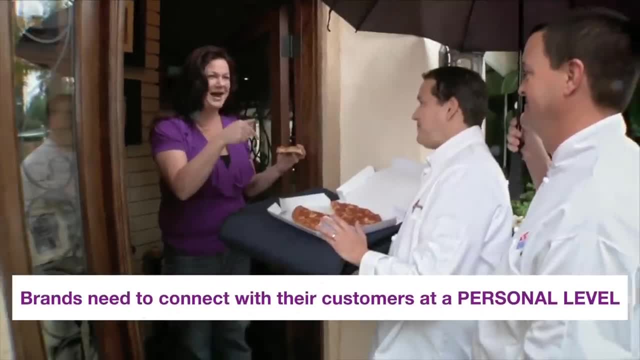 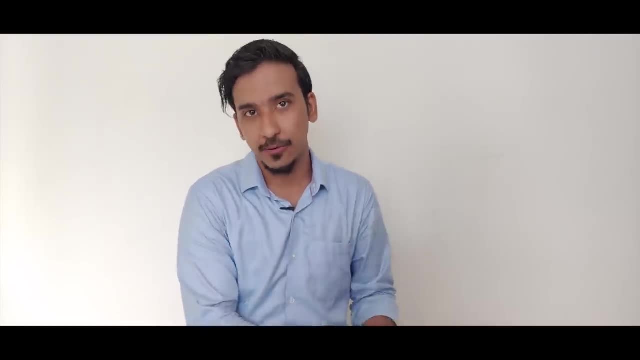 at the end of the day, the brand needs to connect with its customers at a personal level And, thanks to social media, it has become more easier now than ever. Lesson number 3: The moment the customers realize that they are a part of your journey.